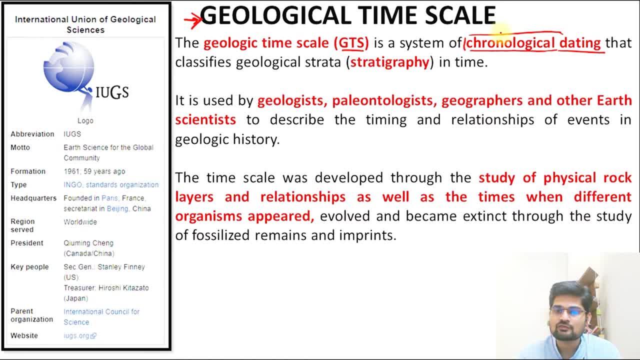 chronology is the sequence, So in sequence of time we date, And the second is the classification of geological strata. that is called stratigraphy. So remember these two important concepts of chronological dating and stratigraphy. that holds key for geological time scale, So it is used by geologists, paleontologists, geographers and other earth. 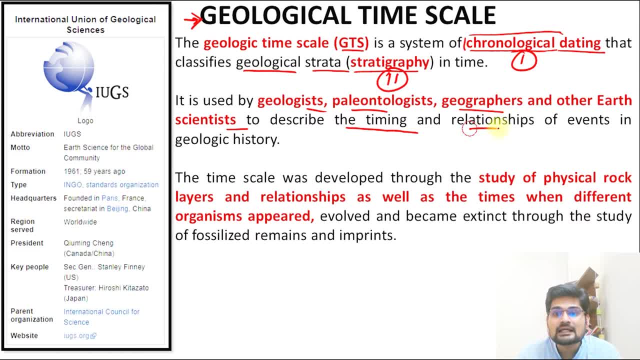 scientists to describe the timing and the relationship of events. So remember, geological time scale is not just about timing, It is about the geological history of relationship of the events that occurred. So that is important. So the time scale was developed through the study of physical rock layers and relationship. 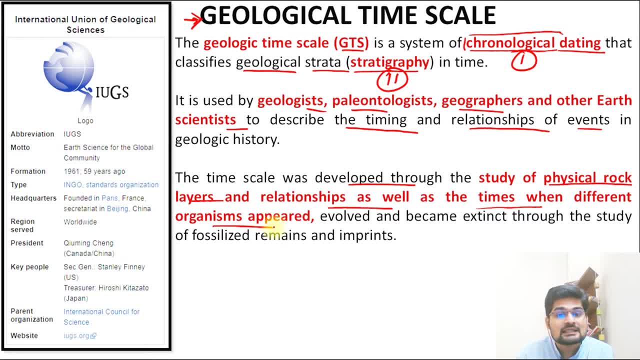 as well as the times when different organisms appeared. So geological time scale is not just about how rocks formed or how the cratonization happened on the rock surface or the earth surface, but rather it also talks about the interrelational aspects, How the organisms 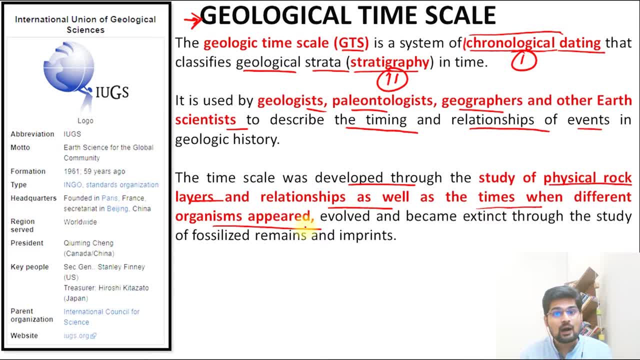 developed how the mass extinctions happened, how the organisms evolved over time period. So these evolution, extinction, all those fossilized remains and imprints, all are the parts of geological time scale that is important. So what we see here is international union of geological sciences, which is the apex. 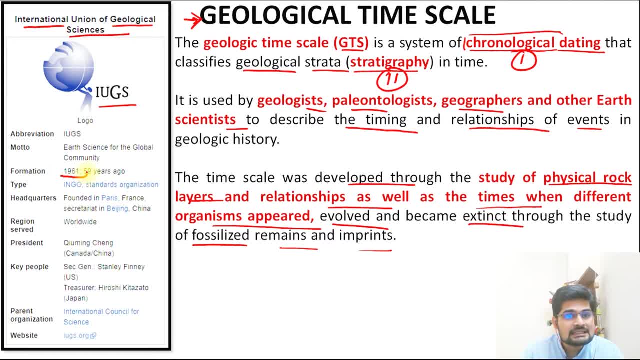 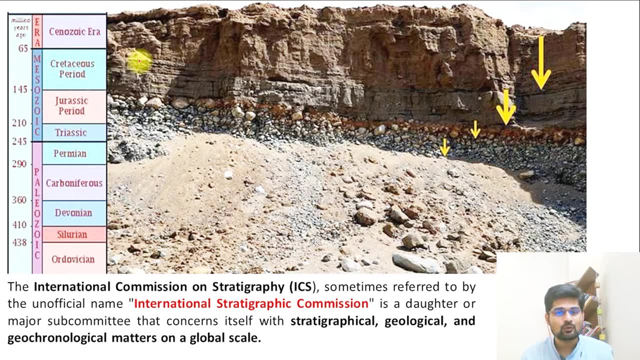 body we see. So this was formed in 1961. that we see- And this is important In terms of what we say- is the creation of this geological time scale. So now, when we talk about stratigraphy, so what comes into your head? what kind of picture? 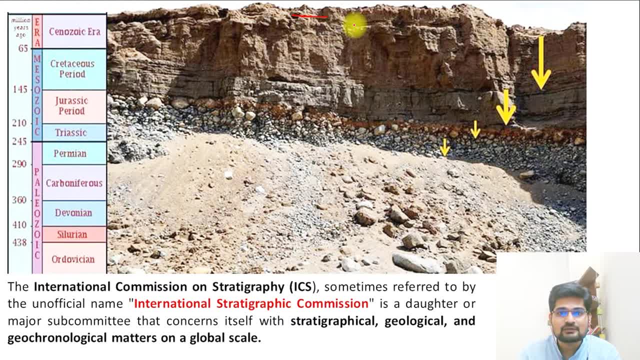 So this is one of the pictures that you can see from the field that was taken in Ladakh. So what you see here is various layers of sediments of different time periods, right? So what we see here is that, from the modern era to the earlier era, what we see different. 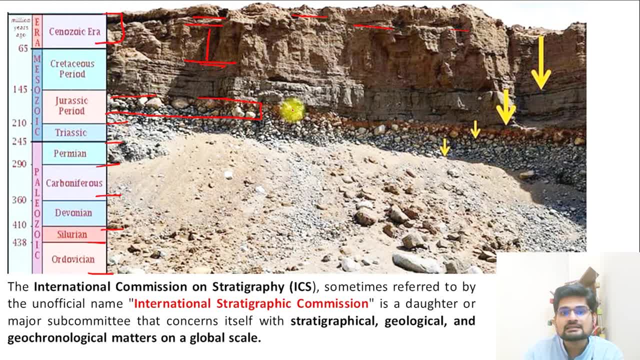 periods and different time periods having various layers in the surface of the earth. So this is what we call as stratigraphy. And who does stratigraphy? The International Commission on Stratigraphy, that is ICS, sometimes referred to by the unofficial name as well, that is, International Stratigraphic Commission. 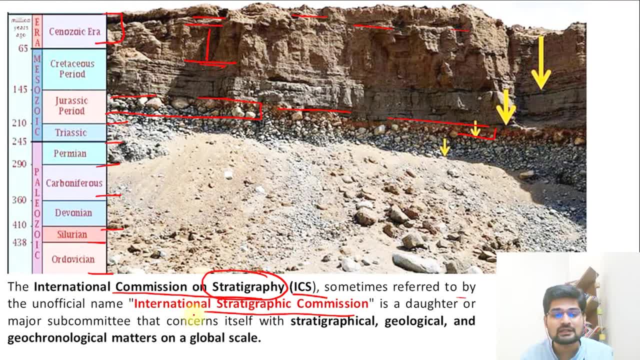 And this is the daughter organization or the subcommittee of what we understood as the International Union for Geological Sciences. So this is the daughter organization or the subcommittee of what we understood as the International Union for Geological Sciences. So that is what is responsible for the stratigraphical, geological and geochronological matters. on, 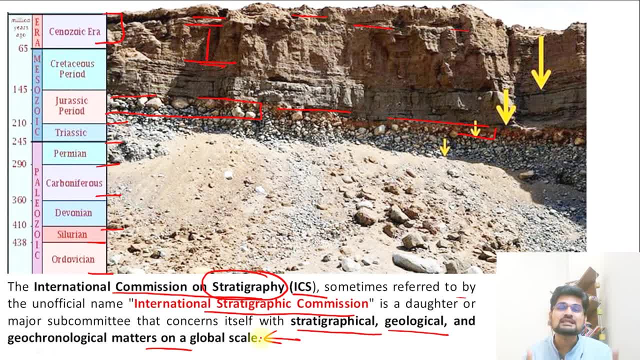 the global scale. So if you have this question, that who decides these times? it's basically this International Commission Stratigraphy and also the EPICS body, that is, International Union for Geological Sciences, which is the part of International Science Council. So now, if we look at the geological history, let me say 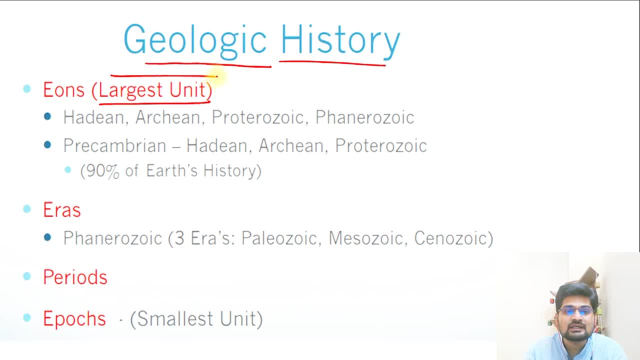 So, first of all, the largest unit of that history is called eons, So that is the first thing to remember. So what is an eon? It is the largest unit of the geological history. So eons, the example, can be Hadean, Archean, Proterozoic and Phenerozoic. 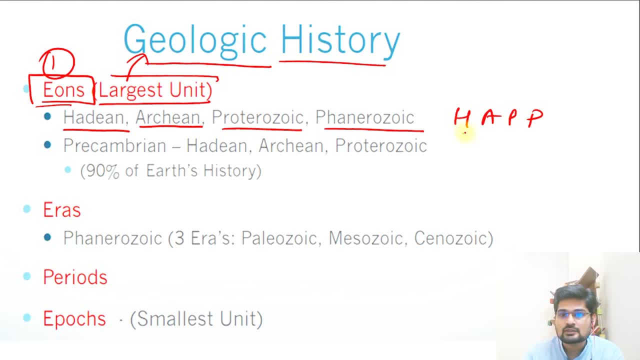 So if you look here, it is H-A-P-P, So if you see here, it is Hadean, Archean, Proterozoic and Phenerozoic And then. So in this Phenerozoic, which is the most recent of these eons, most important is the 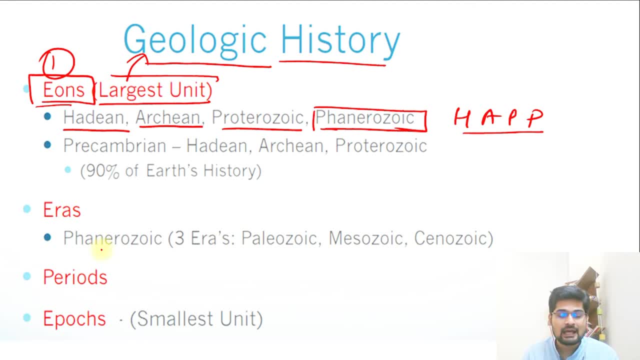 further eras. So they will be studying eras as well. and in the eras, when we say eras, what is there? Example is Pleozoic, Mesozoic and Cenozoic And scaling it down further: in one era there are various periods and in one period there. 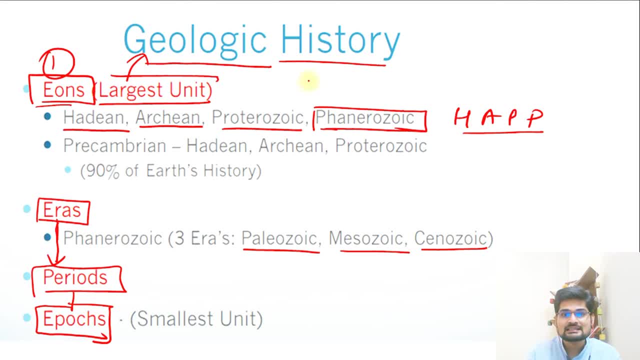 are various epochs. So what we see is, this is one classification of geological history, In which the larger unit, or the largest unit, is the eons, under which there are several eras, under which there are several periods and under which there are several epochs. 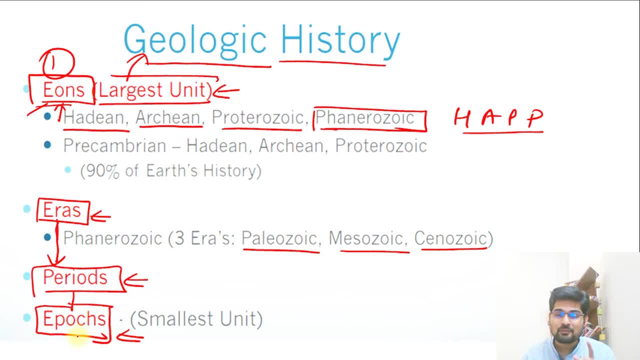 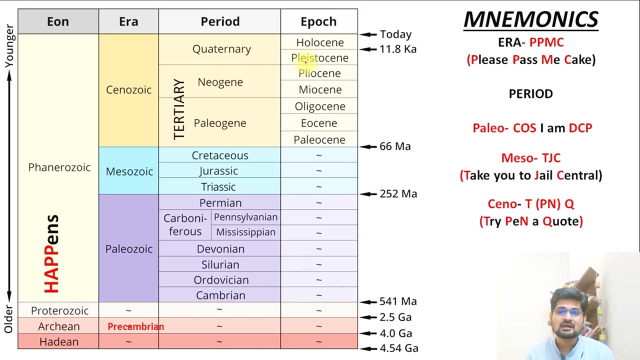 So eon era period and epoch, But remember, under one epoch there is also something called age, So we are going to elaborate it further today. So now the question arise that how can we remember this table? It has so much of information. 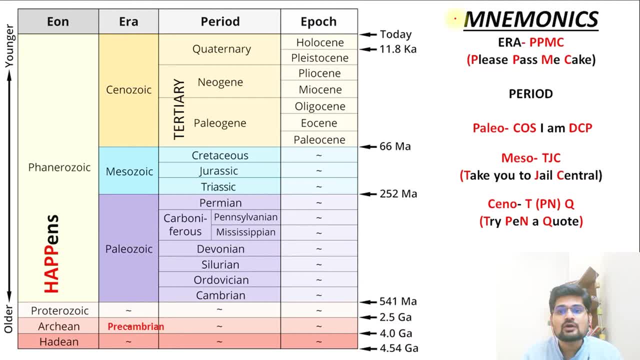 So what is that method? So let's understand something called mnemonics. Now you'll ask me that, what is mnemonics? So mnemonics is one of the important methods of training ourselves, training our brain to remember something in an easier format, a format in which our brain understands comprehensively. 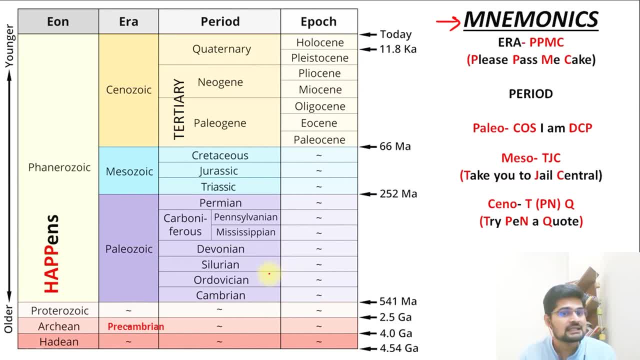 So this is called mnemonics. So we are going to learn some mnemonics and understand the making of this geological history that we study under geological time scale. So first thing, the oldest one that we say is the eon. So what is the first thing? 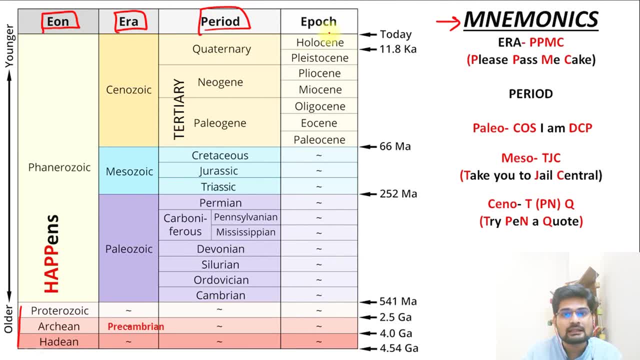 Eons, then what we have era, then we have period and then we have epoch. So this is one sequence that we see. So eons, eras, periods and epochs. So this is one sequence. Now, what we see here is the oldest of this, eon. 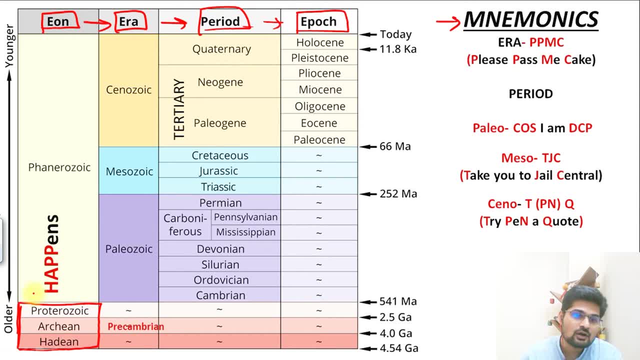 So that is called what we understand as the oldest eons. So the oldest eon is together known as the pre-Cambrian part, So which was before this, Phenerozoic, what we see. So what are those? Hadean, Archean, Proterozoic. 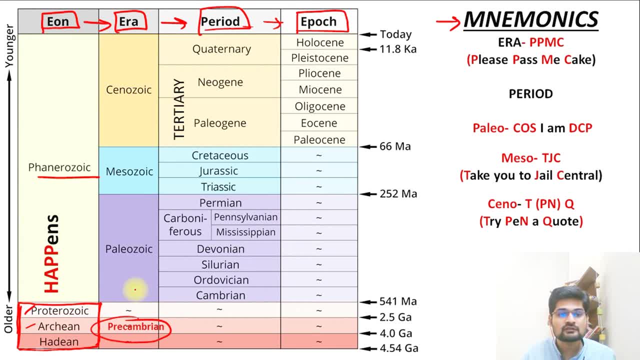 So Hadean, Archean, Proterozoic are together part of the pre-Cambrian times And what is part of the Cambrian So which is after this Proterozoic. So in shortcut, in mnemonics, if we want to read this or remember this, remember this. 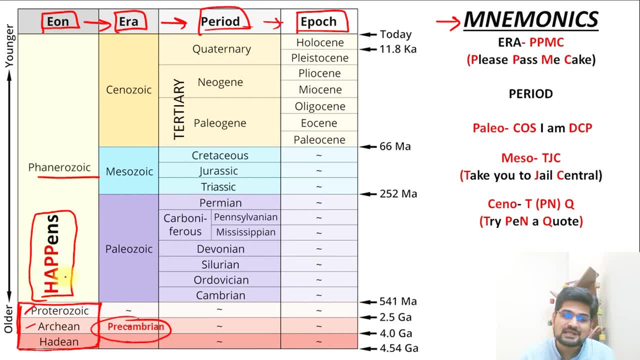 word happens. What is here Happens. So what is happens? H-A-P-P. So what we see here is Hadean, Archean, Proterozoic and Phenerozoic. So just add E-N-S. 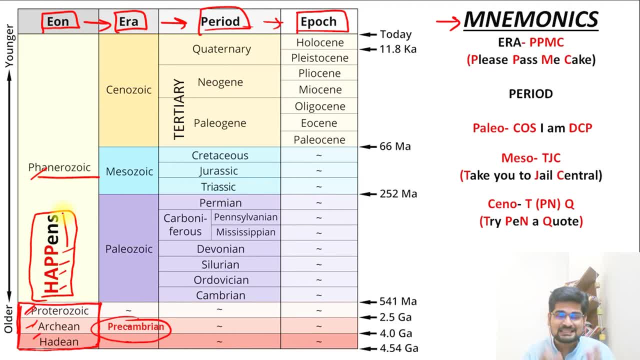 So it happens. So this is one way to remember this: the eons. Now let's go to the next one, that is the era. So how can we remember these eras? Remember, all the eras that we study here are part of this Phenerozoic, that is, the recent. 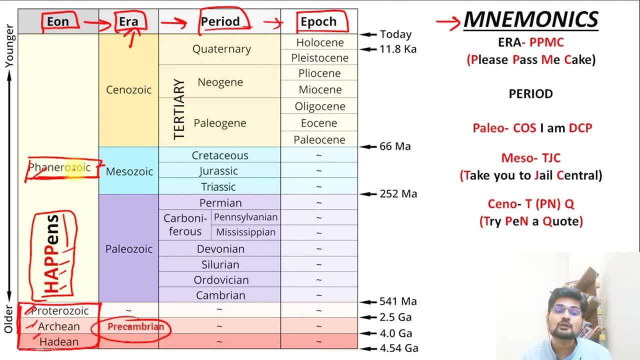 times So recent means that it is present. It is not part of the pre-Cambrian, it is part of the Cambrian now. So in Cambrian what we see is the Paleozoic, Mesozoic and Cenozoic three eras. 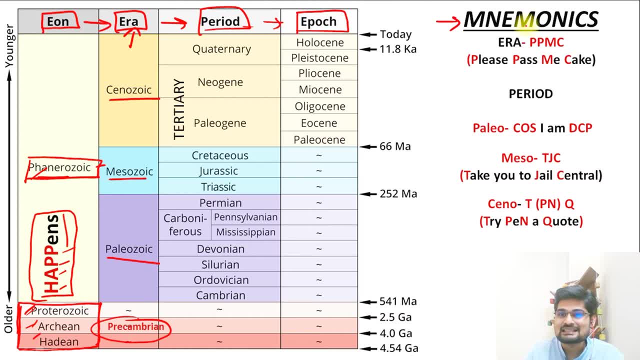 So how can we remember these three eras? Remember this: See, it's P-P-M-C. So what is this P-P-M-C? So one is, what we see is the pre-Cambrian right. The second is Paleozoic, then we have Mesozoic and then we have Cenozoic right. 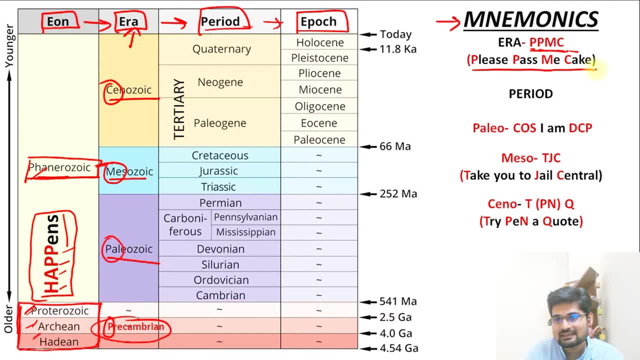 So how can we remember this P-P-M-C By this statement that is, please pass me cake. So as you ask your friend to pass cake to you, so please pass me cake. So remember P-P-M-C. So what is that? pre-Cambrian, Paleozoic, Mesozoic and Cenozoic. 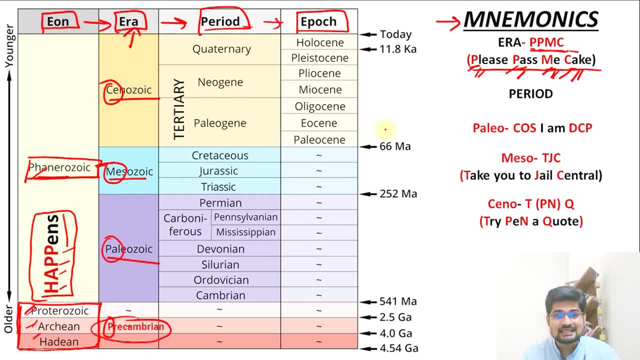 So this is one small statement. This is what we call mnemonics. The second, the next one, is what we call is periods. So periods are part of the one larger era. So what do we see here is Paleozoic, having several periods, right from Cambrian to the Permian, isn't it? 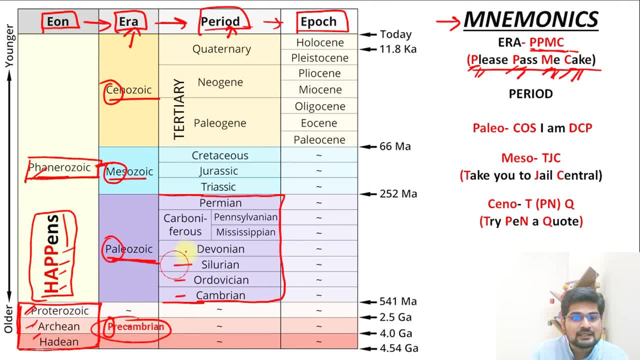 This entire segment, So Cambrian, Ordovician, Silurian, Devonian, Carboniferous, which is further subdivided into Pennsylvanian and Mississippian, and then Permian. So how can we remember these periods? 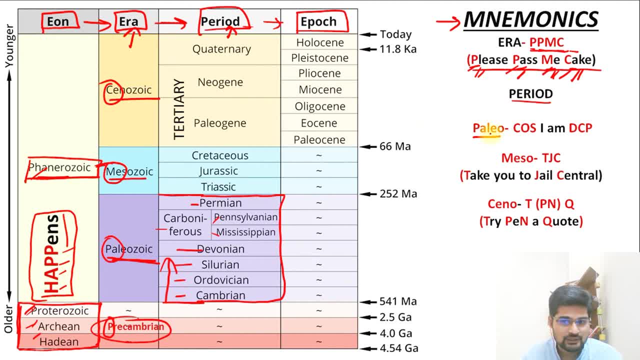 Now remember what we have in the periods is Paleozoic, right And under Paleozoic. what we see here is: there is a statement, cause DCP. So what do we see here? There is a statement, Cause DCP. 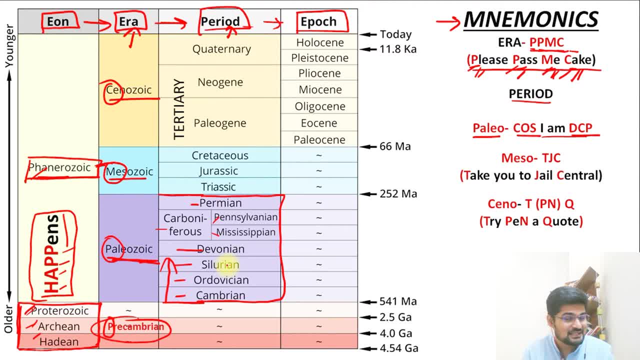 So cause I am DCP. So, if you see, because I am DCP, So this is one statement. So what is this cause I am DCP, Remember? cause is Cambrian, Ordovician, Silurian, So this is what you have. is cause, right? 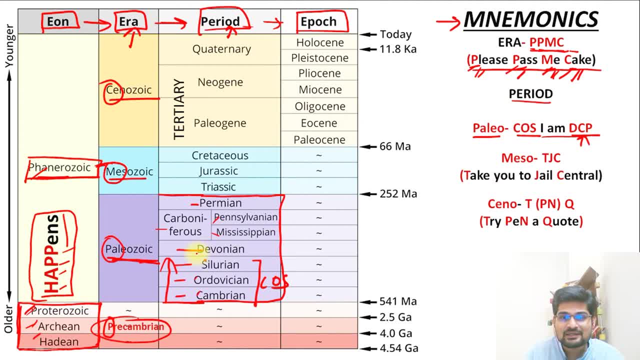 And then what we have is DCP. So what is this DCP? Devonian right, Carboniferous and Permian, So DCP. So in Paleozoic era, how can we divide it into periods Using this particular statement of cause? I am DCP. 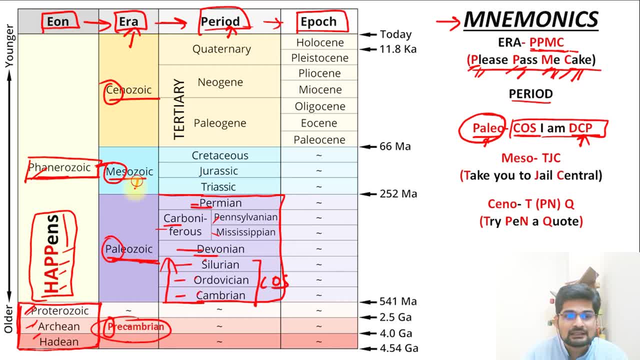 So that is one way to remember. Then, going to the next one, that is, Mesozoic era, we have three: Triassic, Jurassic and Cretaceous. So it is TJC, right? So what is this TJC? You can make a sentence out of it. take you to jail central. 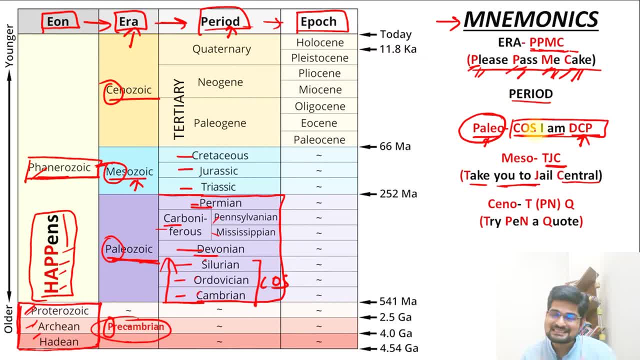 So earlier it was cause I am a DCP. So if you want to remember in sequence, it is cause I am a DCP, I'll take you to jail central. So that is a way of forming a sentence, right. So, Paleozoic, cause I am a DCP. Mesozoic, take you to jail central. 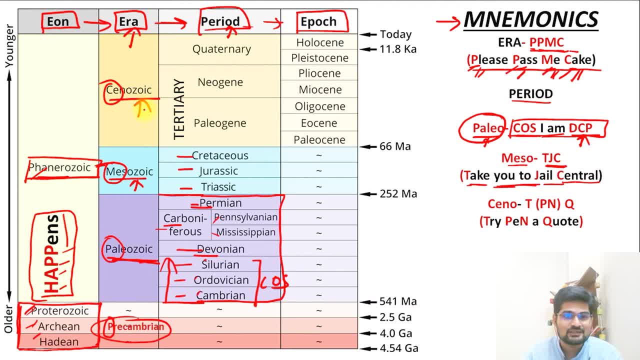 So you can remember it like that. Then what we see is the Cenozoic. So in Cenozoic what we see here is Neogene and Paleogene. These are part of the tertiary period, and then we have the quaternary period. 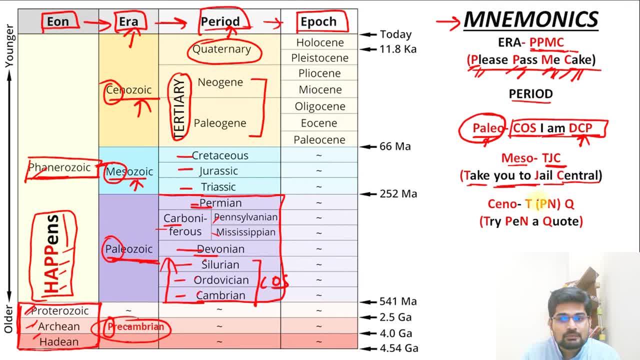 So largely, what is there? It is TQ, but in bracket we have PN right, Because it is Paleogene and Neogene period, So tertiary period. So tertiary is of two types, that is Paleogene and Neogene. So it is TPN, bracket Q: 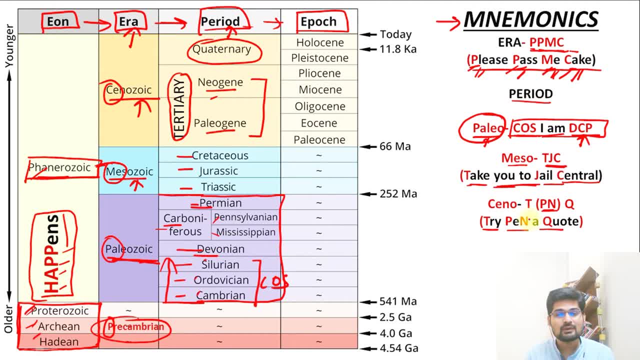 So what is that? Try pen a quote, So remember when you quote something, so this is one statement which you can remember. So try pen a quote. So that is what we have: tertiary, in which you have pen. So that is in bracket. if you want to remember this, pen is your Paleogene and Neogene and 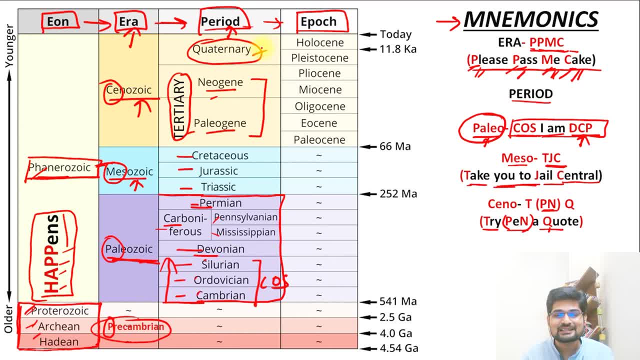 quote that is Q, So quote is basically quaternary. So that is how you remember the periods in Cenozoic era. Now let us go ahead and learn about the fourth one, that is the epoch, the youngest one. So we have several epochs. 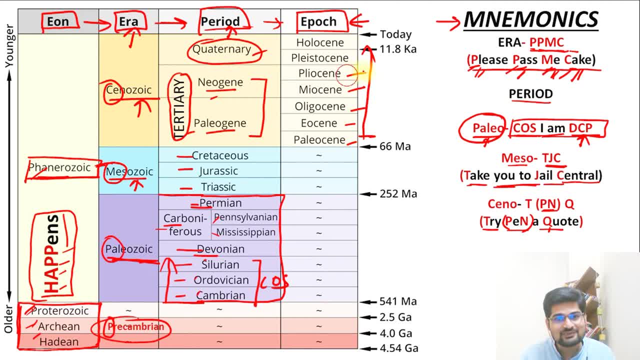 Looking here. So Paleocene, Eocene, Oligocene, Myocene, Pliocene, Pleistocene, Holocene. so how will you remember this? So we are going to learn further the details of what happened along all these eras and 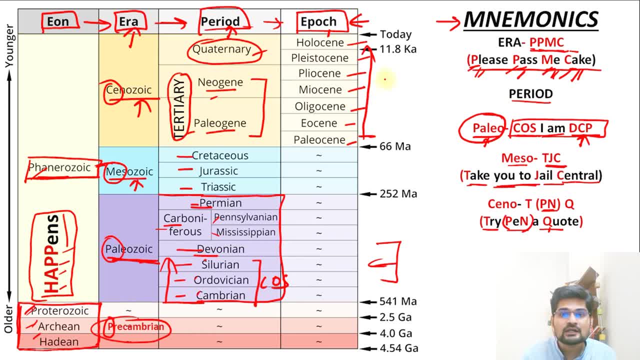 periods, And the 2nd one is called the Epoch. Okay, epoch, we'll be also making a mnemonic of this particular epoch as well, So let's go ahead and learn, one by one, what happened from the beginning. So the first thing that we see here is the eon. 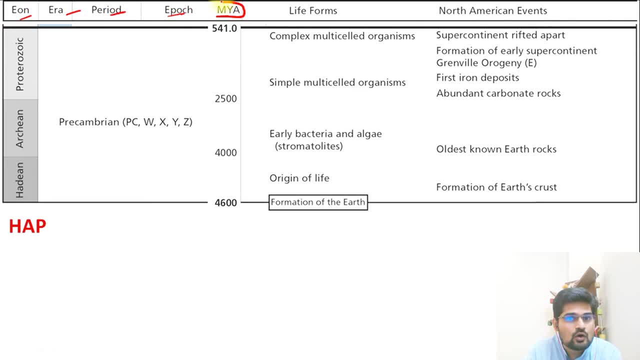 the era, period, epoch. So that is what Million years ago M-Y-A. So what we see is Hadean, So roughly, what we see is the formation of earth. that is, 4.6 billion years ago, remember, So that. 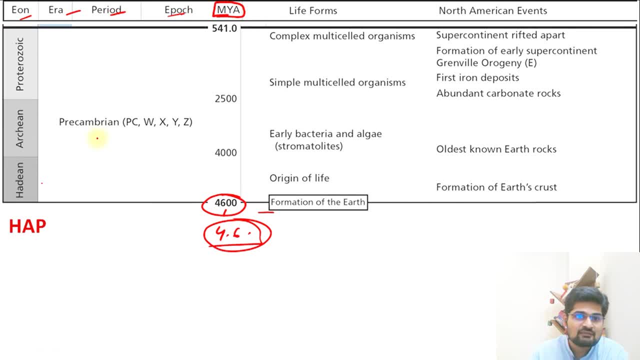 is what? 4,600 million years right. Then what we have is the Archean- that is the next segment- roughly 4,000.. Then what we have is the Proterozoic, roughly 2,500.. And then what we see is: 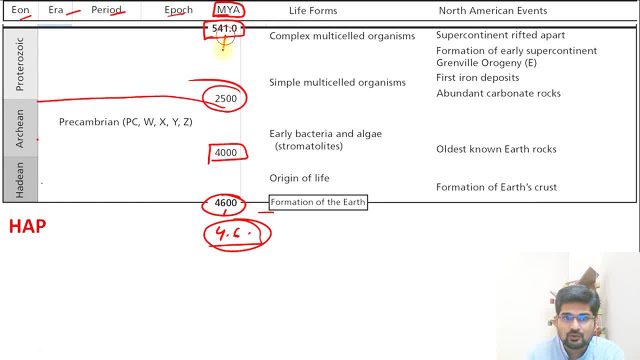 about 541 million years ago. remember From 2,500 to 5. So 541 million years ago. what we see is this demarcation where now this Precambrian ends and the further Cambrian, that is, the Necrophysicists are formed. So that is what we have here. So that is what we see is the. 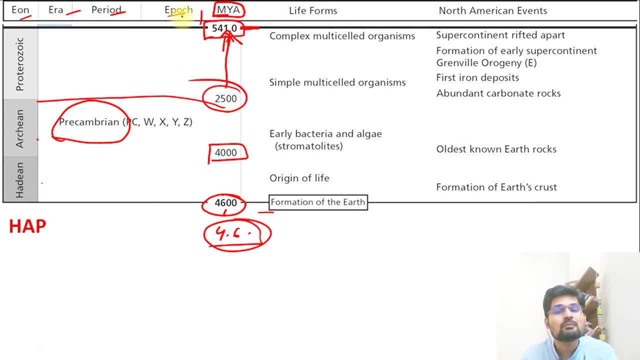 Necrophysicists are formed. So that is what we have here. So that is what we have here. So that is. next. Phenerozoic segment starts. So what are the developments that we see here During Hadean? the origin of life is here, right? So formation of earth crust is there Then. 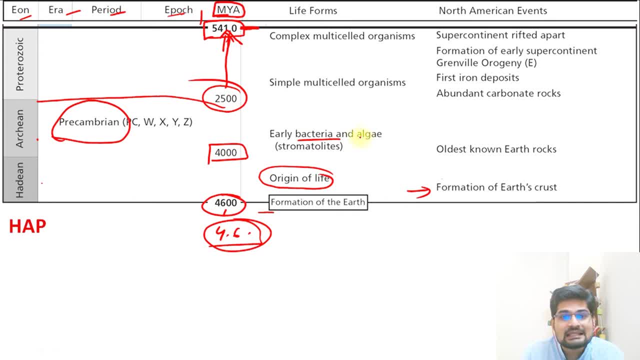 what we see here is in Archean, we have bacteria and algae formations. right The earliest known earth rocks are there. Then what we see here is further in Proterozoic, we have simple multi-celled organisms, So from single cell bacteria to multiple cell bacteria organisms. 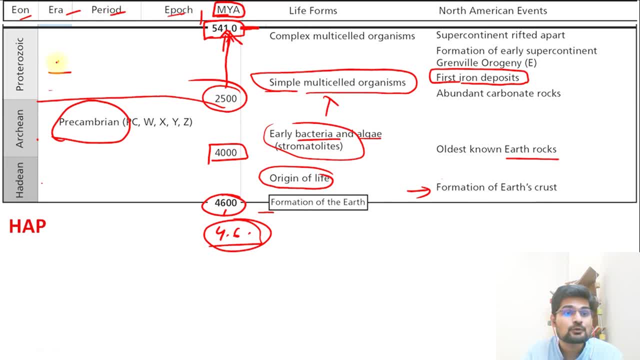 first, iron deposits have been found to be of Proterozoic times, right Abundance of carbonate rocks, Then further supercontinent which was formed for the first time was part of this particular time period, And then complexity increased with evolution. So complex, multi-celled. 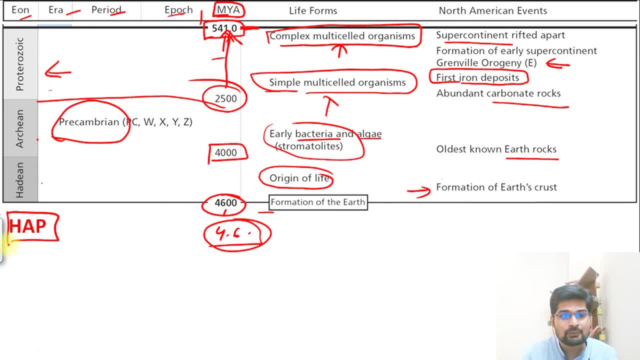 organisms developed. So what we see here is this: in this HAP, right From 4600 to 4000, right To 2500 and then 541.. So this is the demarcation line And these are the developments that happened during. 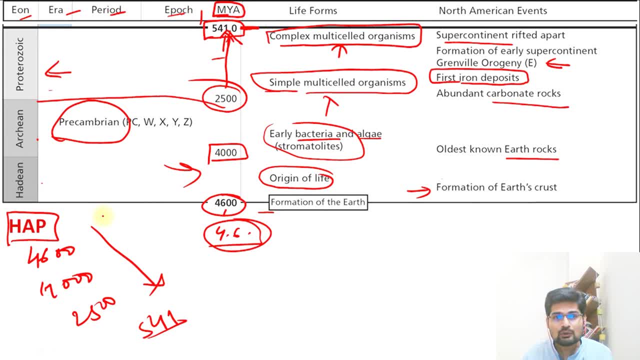 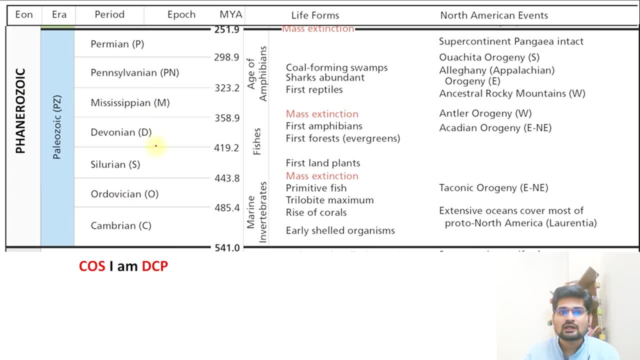 this particular segment of the eon. right Now let's go ahead into Phenerozoic eon and understand the eras so that we have to learn further. So now coming to this Phenerozoic, the first era, remember that is Paleozoic, right? So 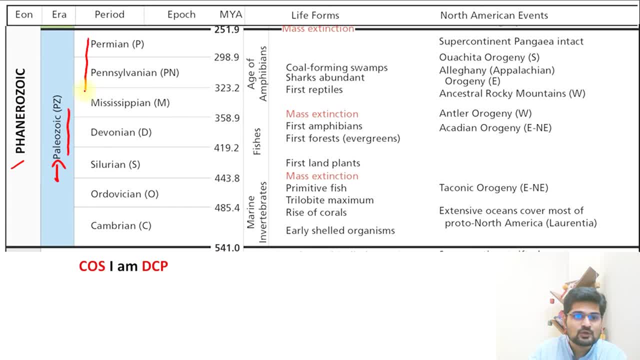 under Paleozoic. what we see is these periods, so many periods, as we have classified by this particular mnemonics, That is, Causiamer, DCP, So COS, DCP So Cambrian, Odovician, Silurian, Devonian and 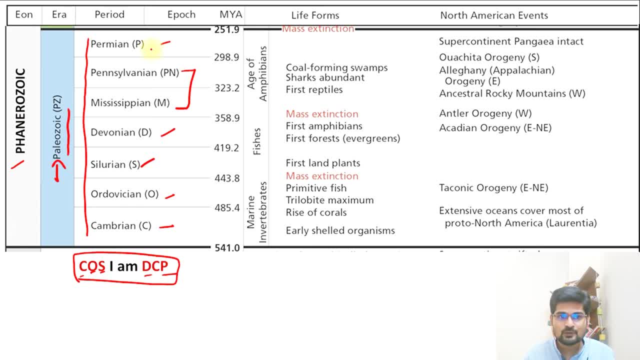 this is part of Carboniferous and then Permian. So now we need to understand what is mass extinction from this particular point. So what happened? From 541, we start going further ahead and we see marine invertebrates now in this situation, 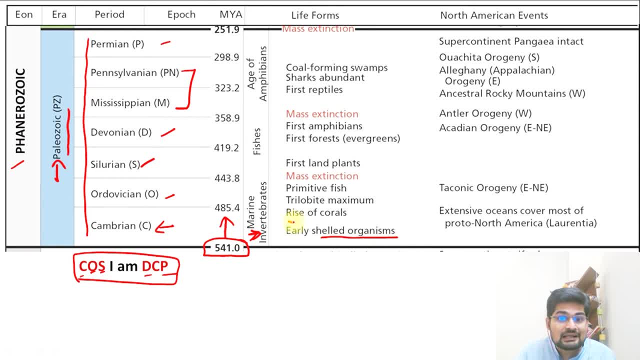 in Cambrian We see early shell organisms, rise of corals. So now remember, corals are part of Cambrian right. So C for coral, C for Cambrian, if you can remember that, Then primitive fish and trilobites, So this is part of Odovician right. Then what we see is during this transfer, 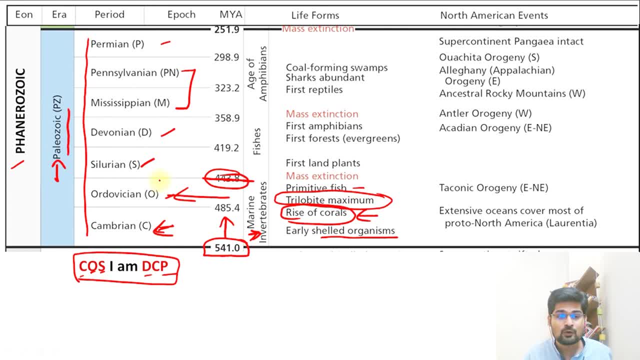 during this change, during 443 million years ago. what do you observe From Odovician, this Silurian time? that change was through this mass extinction. So that is the first mass extinction between what Between these O and S of COS, So COS. 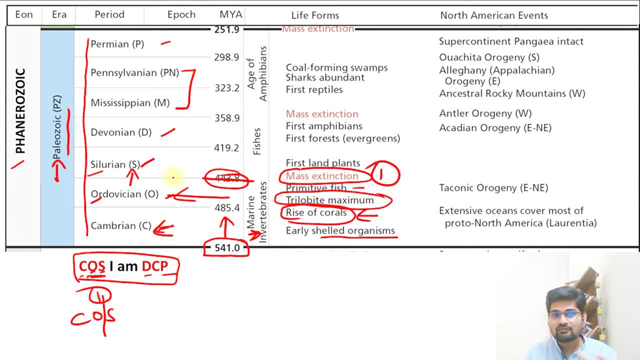 so this is where the first mass extinction is, there right. Then further in Devonian, what we see, First forests, which are evergreens that we know, Then first amphibians come in, So fishes and amphibians. what we see here, further in Devonian, Then again from Devonian, 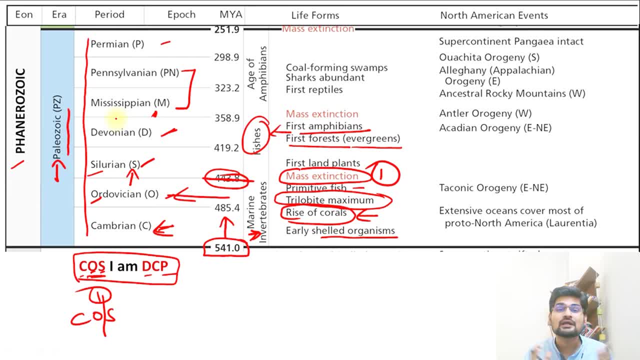 to this Carboniferous, where you have large parts of the Carboniferous. So this is the first mass extinction. So this is where the first mass extinction is. Then, further in Devonian, the carbon, the coal extract now coming out, So carbon is named from Carboniferous right. 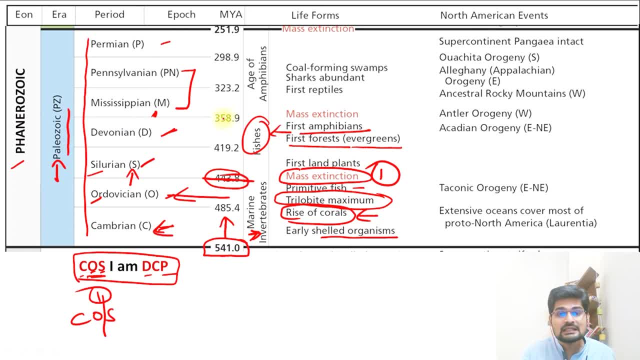 So Carboniferous was that particular time which accompanied this particular mass extinction. number two right So between Devonian and Mississippian. So if you say between the upper and lower Carboniferous, So remember this is lower Carboniferous, then this is. 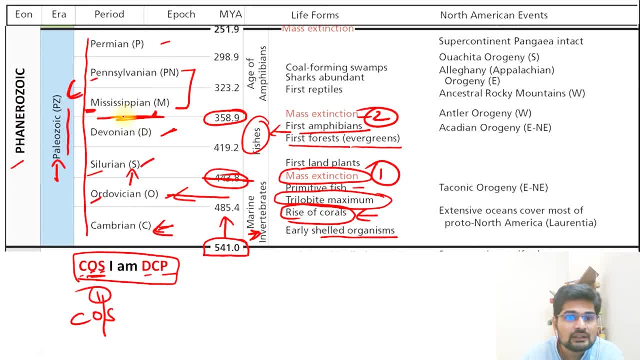 upper Carboniferous. So what happened Mississippian and Devonian in between them during this particular million year, that is 358.9.. So almost 360 million years ago there was the second mass extinction. that happened. 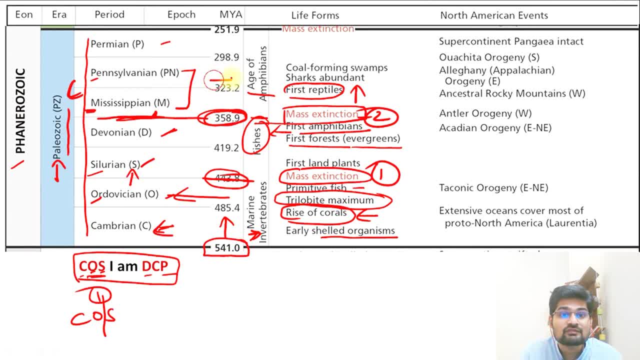 So first reptiles come in during this Carboniferous time, right Then coal forming, swamps and sharks abundant. So what we see is the maximum coal formation during this particular time period of Carboniferous period. So the next part is from about 300 to 251.. This is called Permian. 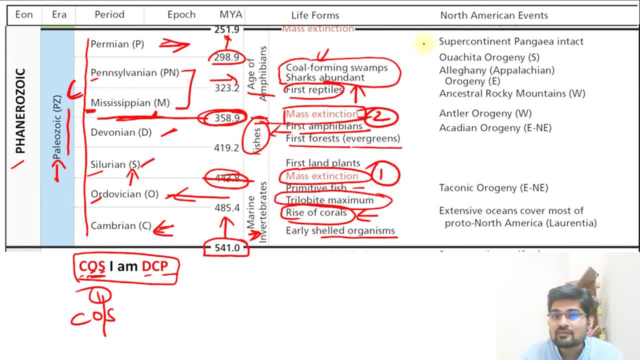 Remember the Permian was that particular phase where we find this supercontinent. So remember now Pangaea was formed at that particular time, which is Permian. So Pangaea and Permian PP, you can remember like that. And then again, at the end of Permian, about 251 million years. 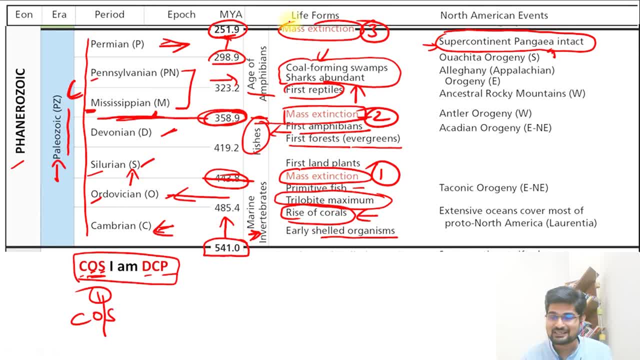 ago there was this third mass extinction again. So this is the three mass extinction in Phenerozoic first era, that is, Paleozoic. Now we are going to Mesozoic further. So now let us go ahead and learn Mesozoic. 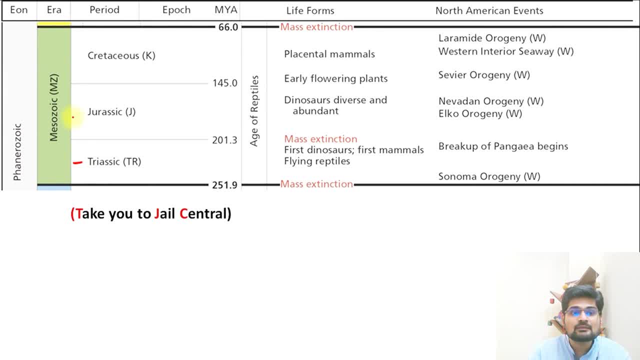 So in Mesozoic, what we see is these three important periods, What is that? Triassic, Jurassic and Cretaceous, right, So T, J, C, So that is what. Take you to jail central, because I am a DCP, remember. So take you to jail central. So 251.9,. that is another. 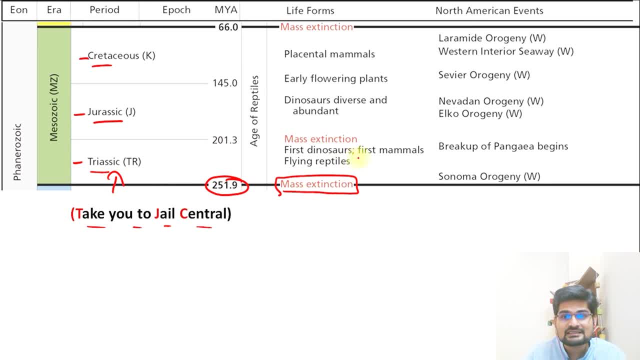 mass extinction coming into the Triassic, then first dinosaurs, first major reptiles, and again going from Triassic to Jurassic, So about 200 million years ago. there is another mass extinctions. So this is mass extinction number three that we know, and this is mass extinction number four. So this is: 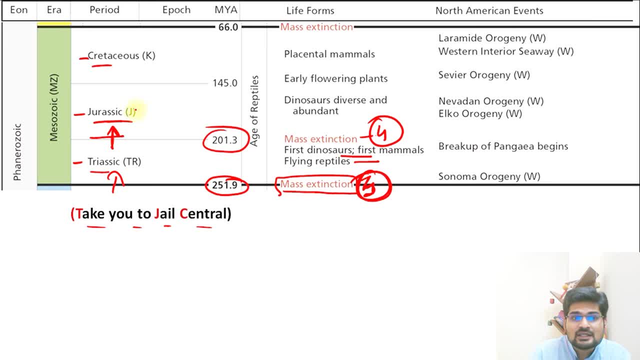 fourth, mass extinction, that further we go into the Jurassic age. So you remember Jurassic Park. you must have seen the movie The Age of Dinosaurs, very famous. So dinosaurs and diverse further flowering plants and other reptiles that we find in this particular time. period, reptiles. So if you are being asked about the question, that which is the age of reptiles, remember, Mesozoic is the age of reptiles, largely the Triassic, Jurassic and Cretaceous. Further going from Jurassic to Cretaceous, what do we observe? The placental mammals for the first. 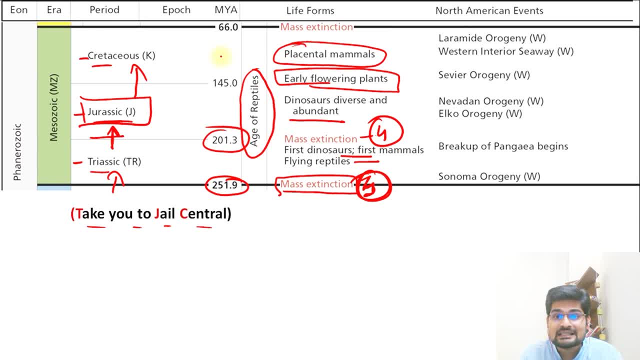 time. So those mammals which carry their children in their womb, there is an attachment in placenta, what we say the umbilical cord. So placenta formation was there during this particular evolution time period and again, what we see here is about 66-65 million years ago. 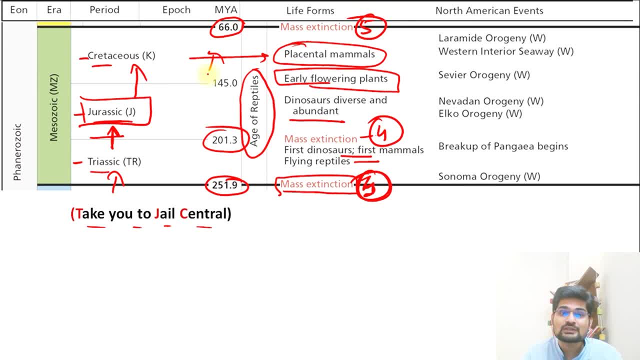 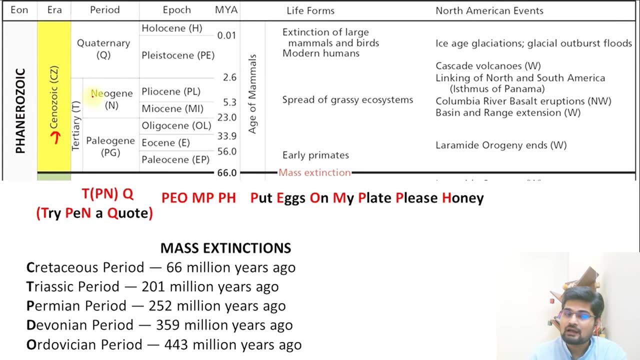 the fifth mass extinction happening. So the age of dinosaurs coming to the end, with this right in the Mesozoic era. Now let's go ahead and look at the most recent era, that is, the Cenozoic. So what we see here is the Cenozoic era. As we know, this is 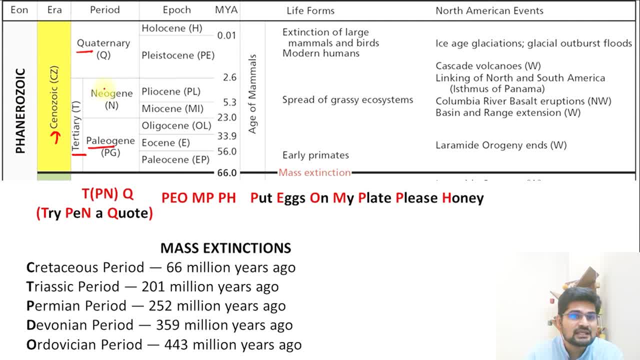 T and Q. So under T we have Paleogene and Neogene. So what we have learned is T bracket P and Q. So try pen a quote. So remember this. Now. what we see here is that after this fifth mass extinction now we see early primates here. So what is important here is the spread of grassy ecosystem. 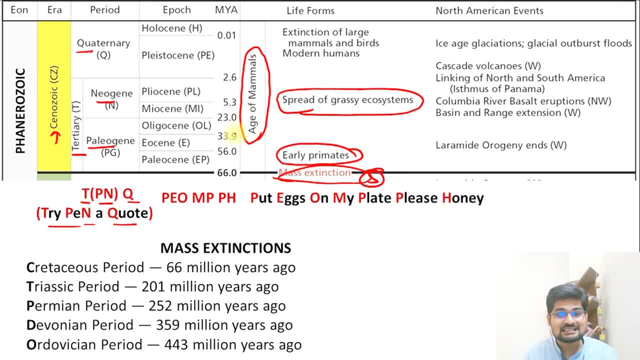 the age of mammals come into the picture. So what we see is the age of mammals, the start of the modern humans come into the picture in this particular era of Cenozoic. So, going from tertiary to quaternary, we find the development and evolution happening and what we see is the 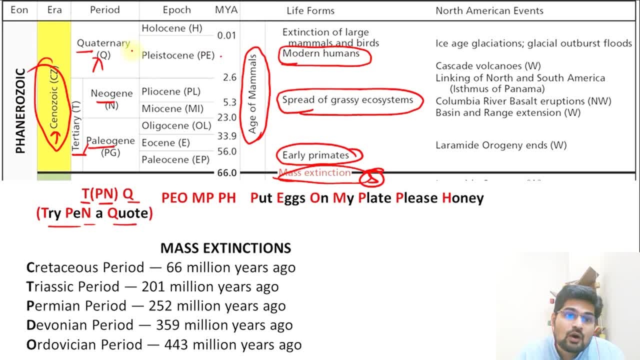 modern human come in the further quaternary period. So under quaternary period, what we have is this particular epoch. What is that? Pleistocene? So remember this. Pleistocene is when what we see is the arrival, The advent of modern humans. But before we go ahead to this epoch, let's understand that how. 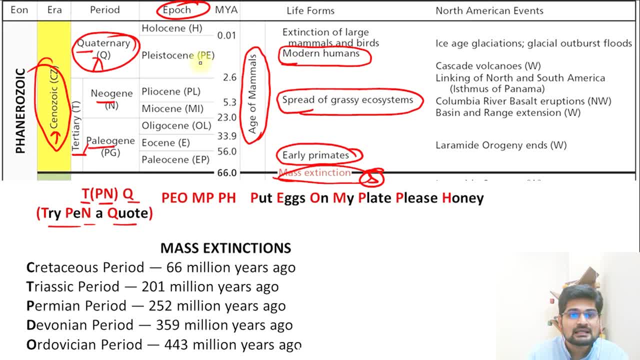 to remember this epoch now. So what we see here is that there are number of epochs in the same Cenozoic era, So that is Paleocene, Eocene, Oligocene, Miocene, Pliocene, Pleistocene and 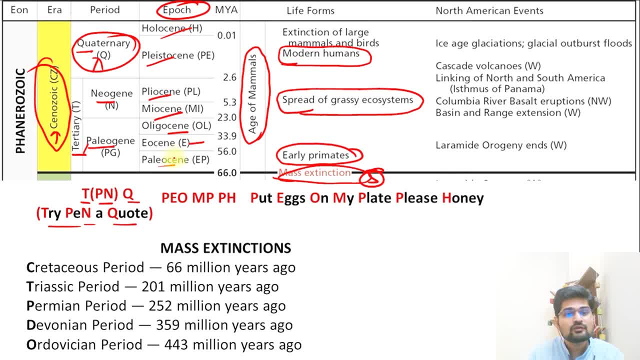 Holocene. So how to remember this? Now, if you make a shortcut, it is P, E, O, M, P, P H, right? So Paleocene, Eocene, Oligocene, Miocene, Pliocene, Pleistocene and Holocene. 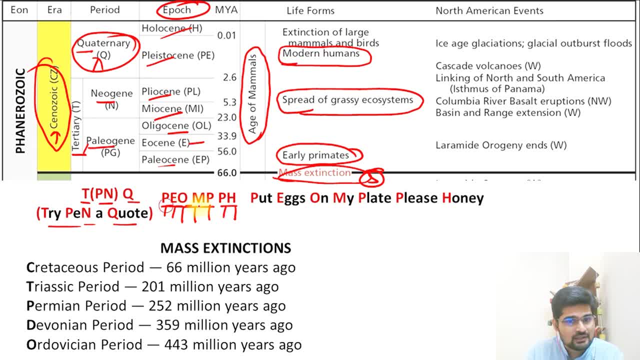 So this is the shortcut Now if you want to form a sentence, it's very interesting: So, put eggs on my plate, please, honey. So a person is asking to his wife that, please, honey, put eggs on my plate. So this is a sentence to remember. so P E, O, M, P, P H. 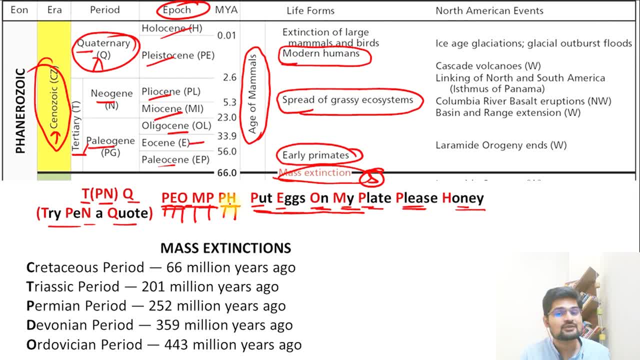 So P E, O, M, P, P H, So that is what? put eggs on my plate, please, honey. So this is how you have to remember. now, going from the 66, that is the time of mass extinction, we are now moving ahead towards the 1 million year mark. 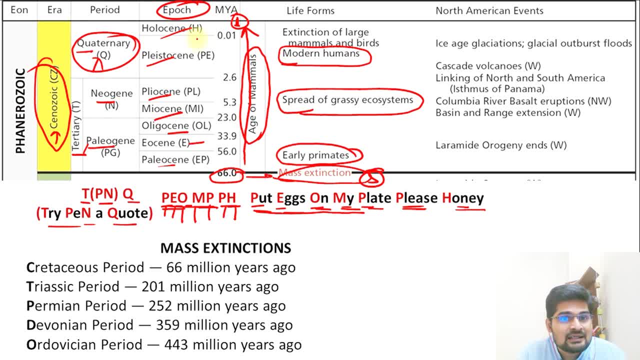 right and furthermore. So what we see here is that the Holocene and the Pleistocene, where we see largely the modern humans, come in and then comes the human history. So when we have learned about the Phenerozoic right, from the Paleozoic to Mesozoic to Cenozoic eras, what we see is number. 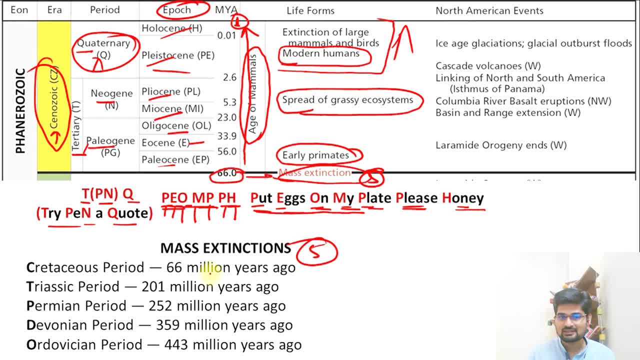 of mass extinction, that is about 5 mass extinctions. So what is that? So remember 443, which was Ordovician, So O. then we have Devonian, that is about 359 million years ago, So 359. then we have Permian, So this is about 252 million years ago. Then we have the Triassic. So going from Triassic, 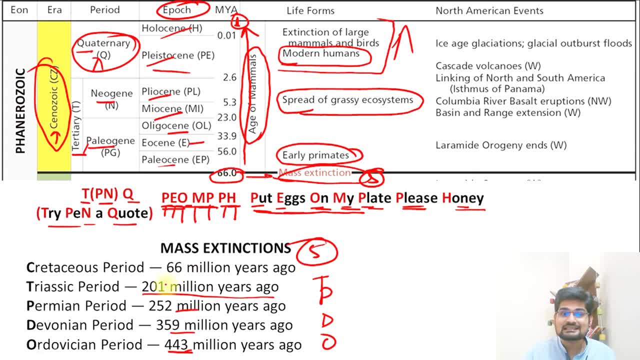 to Jurassic, So that is about 200 million years ago, and then Cretaceous, that is about 66 million years ago. So what we see here is this ODP and TC. So remember this ODP and TC in this particular sequence from 443 to 643.. And now it is. 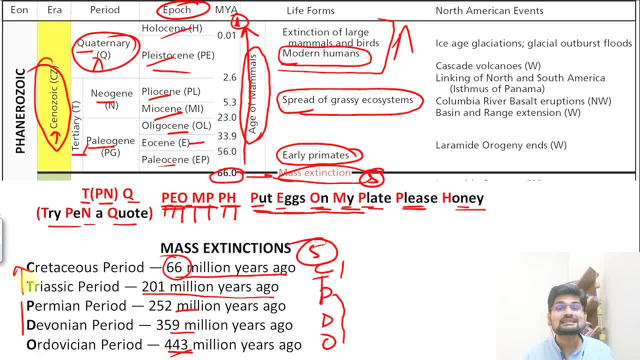 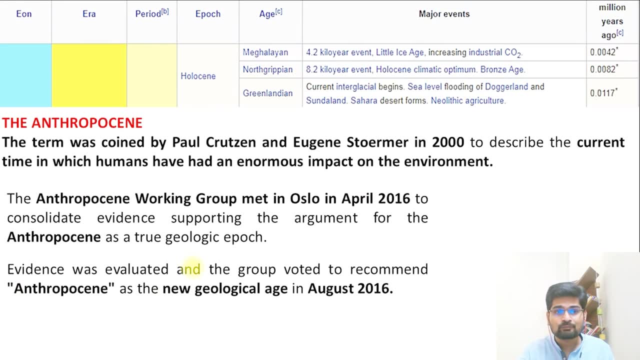 being said that currently we are on going into the sixth mass extinction because of the climate change. So remember, when we say the concept of sixth mass extinction, it is currently happening because lots of species are now being lost. So that is important here. Now another thing that is important in geological: 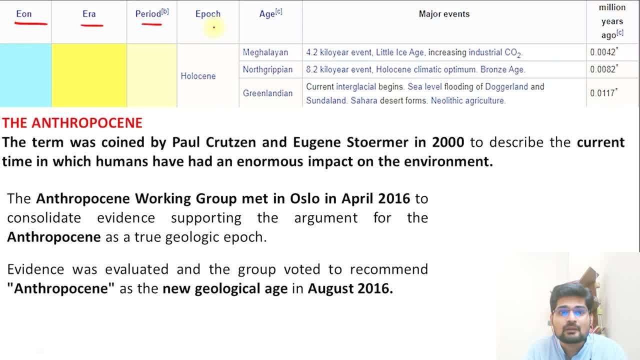 time scale is not the sequence, just Eon Era Period and Epoch, but also this Age thing. So what is this age thing and how did it come up? Remember further, this Holocene has been divided into three different ages, So that is the most recent part, What we see here. 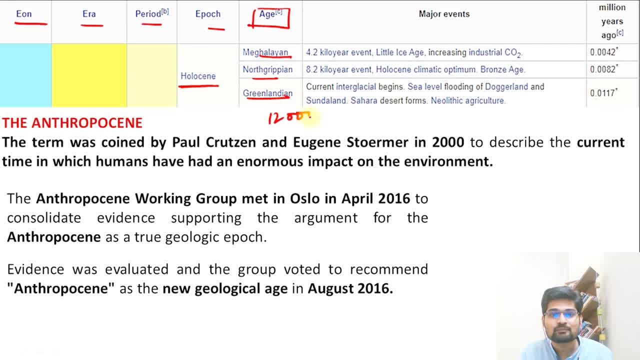 is about the twelve thousand years old history. So remember, right from twelve thousand years, 8200 years ago, to this 4200 years ago in the before Christ time. So that is, what we see is 12000 BC when we say this is the time when we say it is Greenlandian age. What we see here is: 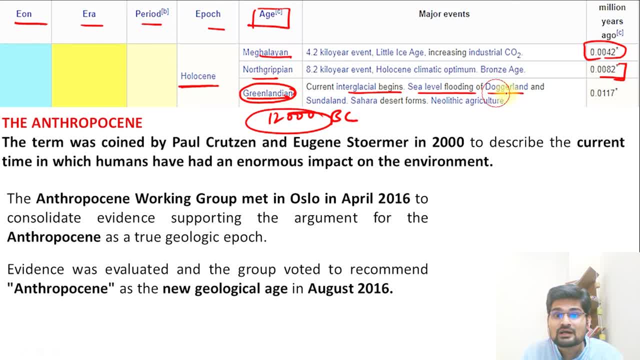 current interglacial begins, sea level flooding of Dogaland and Sundaland, Sahara desert formation happens, Neolithic agriculture starts. So that is about 12000 BC to 10,000 BC. Remember that time. Now next phase was this: 8.2.. So that is about 8200 years before Christ. And what is we say? the 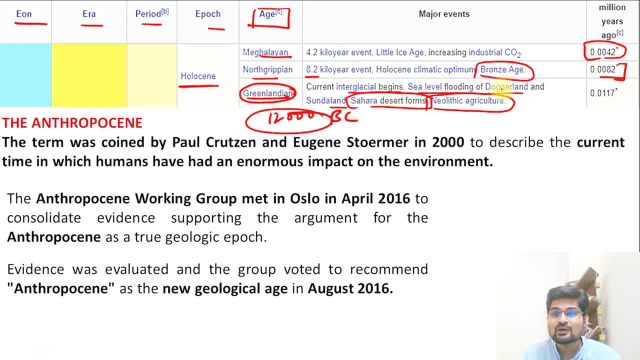 beginning of Bronze Age civilization right. So from Neolithic we go to this Bronze Age that we say So. Neolithic basically means new tools, So that is how it is: Neolithic. So Bronze Age is about 8200 years old and that has been classified as North Grypian, And then further about 4200. 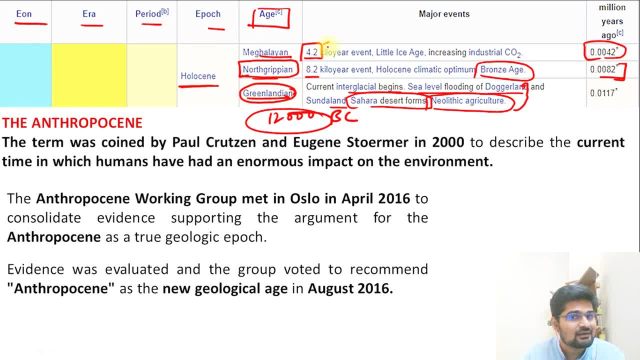 years before Christ, So that is about 8200 years before Christ. So that is about 8200 years before Christ, So that is before Common Era. So 4200 CE, right before Common Era, BCE. This is the time. another demarcation has now recently come up and which has been named after this particular cave. 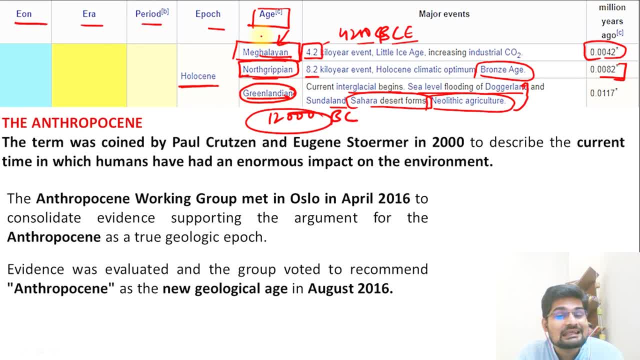 in Meghalaya, we know. So that is why it is called Meghalayan Age. So Meghalayan Age is now currently continuing from 4200 BC to present and going on. So Phanerozoic Eon. then we go into this. 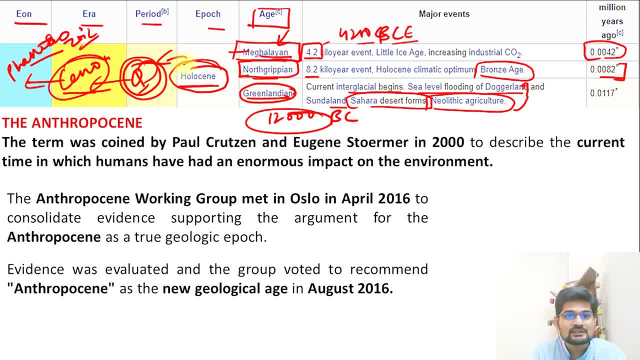 era, which is Cenozoic, then into Quaternary Period, then going into this Holocene Epoch And under this Holocene Epoch, currently we are now continuing into the Meghalayan Age. So that is the particular scaling down of geological time scale. Now there is something. 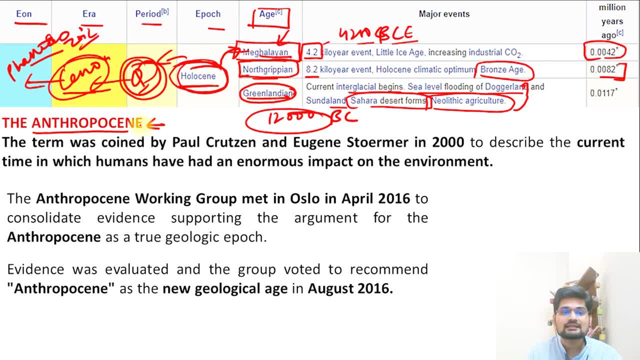 also used in this colloquial term that is called Anthropocene. What is this Anthropocene and how does it come? This term was coined by two scientists, that is, Paul Crutzen and Eugene Stormer, In 2000.. So to describe what The current time in which humans have had enormous impact on the 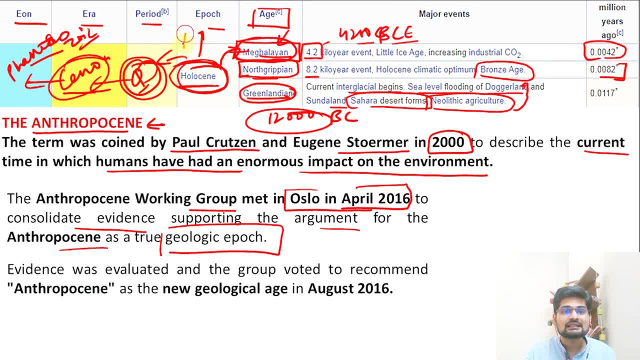 environment. So after Holocene, what we say is that advent of Anthropocene. But evidence was evaluated on the group voting and this was the new geological age, confirmed by the International Agency in August 2016.. So Holocene is not the recent one. now Anthropocene right from the Meghalayan. 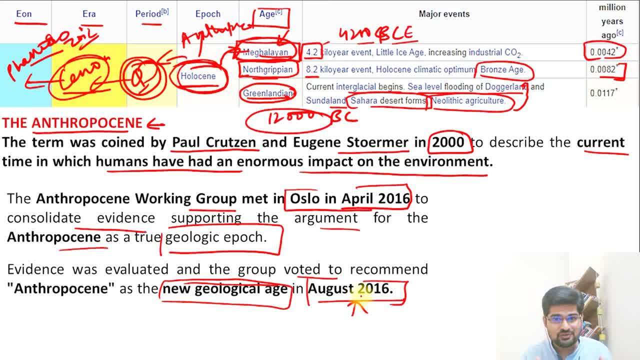 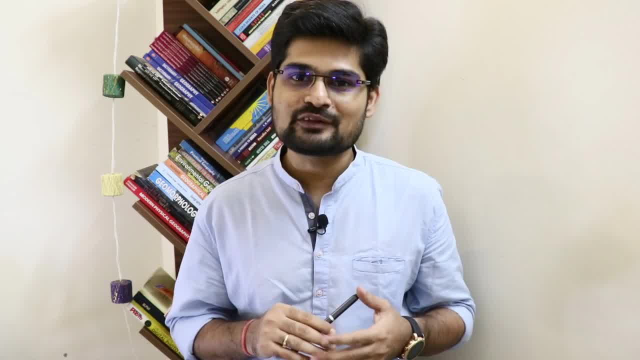 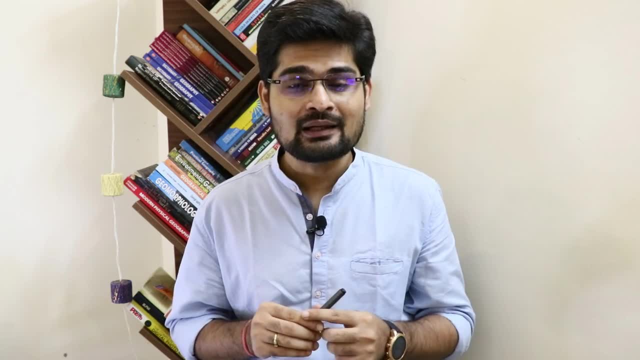 Age is now the current geological time in which we are there presently. So now, when we have learned about the geological time scale, the history of evolution of mankind, as well as various mass extinctions and how to remember it in easy way, I hope you understood it well. So, furthermore,